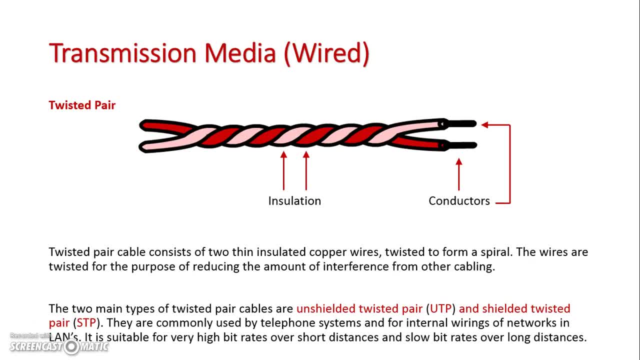 twisted together. These wires are twisted for the purpose of reducing the amount of interference coming from other types of cabling. Now we can see that the actual twisted cables are insulated in order to protect them and reduce interference, and contain conductors on the inside. They're commonly used in telephone systems, as well as internal wiring in network. 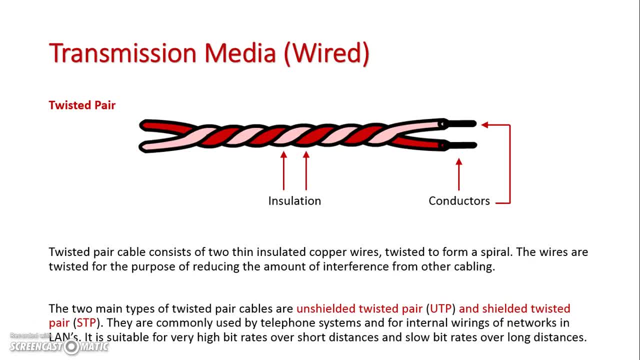 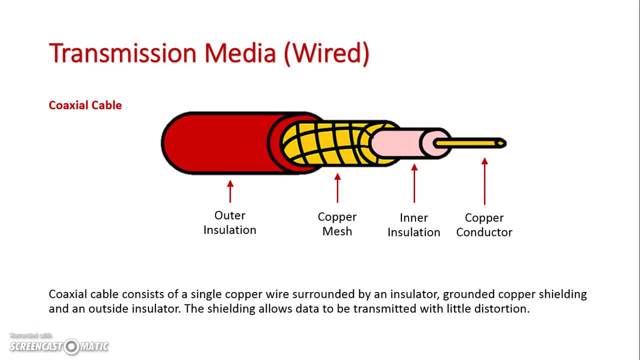 LANs. They're suitable for very high bit rates over short distances, but basically they're cheap and easy to use. The next type of cabling is coaxial cabling and, as you can see here, the copper conductor is very secured. 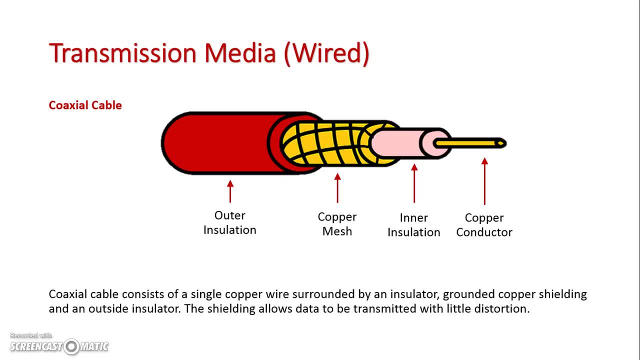 We've got an outer insulation, a copper mesh, an inner insulation and then the actual conductor itself, And so this type of transmission is also used over a short distance, but is a lot more secure and less susceptible to interference. The final type of transmission we'll look at is optic fiber cabling. Here we have covering. 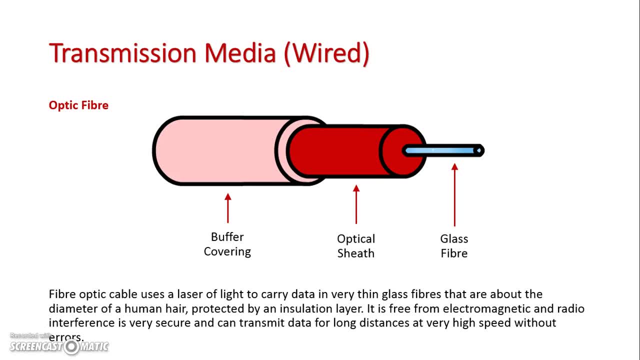 as well as sheath. but instead of having copper conductors, it has a glass fiber which is very thin. This glass fiber runs the actual transmission many times faster than copper ever could, So it uses a laser light going down this glass fiber, which is the diameter of a human. 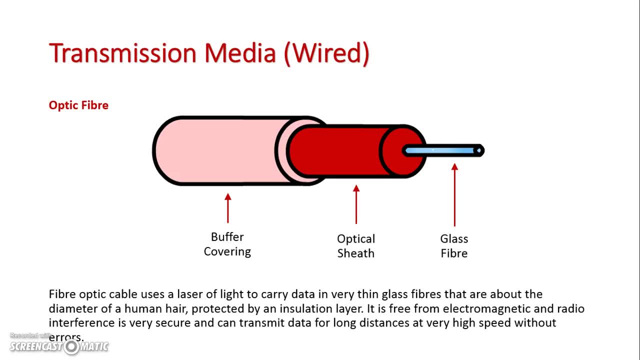 hair. It is free for any type of EMI or radio interference and can go over very long distances. This is the type of cabling they're trying to bring in with the National Broadband Network to increase the internet speed. So let's look at all these types of cables side-by-side and compare them. 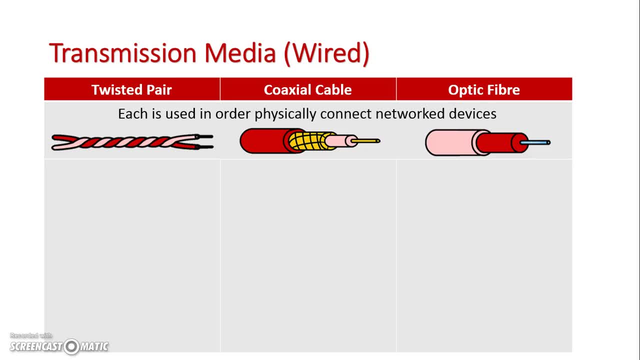 So basically each one is used in order to physically connect network devices. So they're all wide, they're all physical. we can touch this type of transmission media, Both twisted pair and coaxial, have pretty short distances. With twisted pair, at about 100 meters in length, it can go over coaxial at 500 meters. but 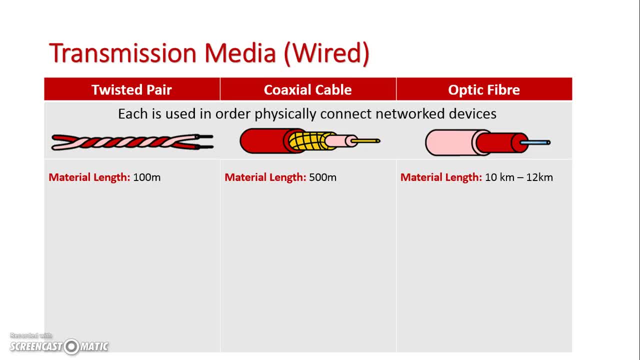 optical fiber we can go to 100 meters in length and coaxial at 500 meters, But we can go to 10 to 12 kilometers running cable. The speed is about 10 to 100 megabytes per second with a twisted pair.